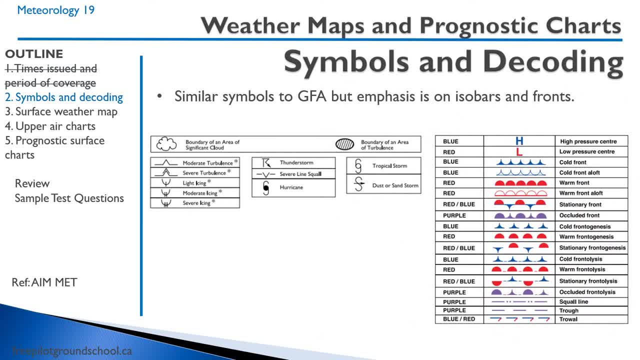 Here are the symbols. They're pretty much the exact same symbols as the GFA, But the emphasis is on isobars and fronts. They're not going to be talking about as much in clouds and things like that Here down at the bottom. So you remember trowel And we have these troughs. remember So an elongated area of low pressure? It's a trough, And so this is what you can expect on these weather maps. 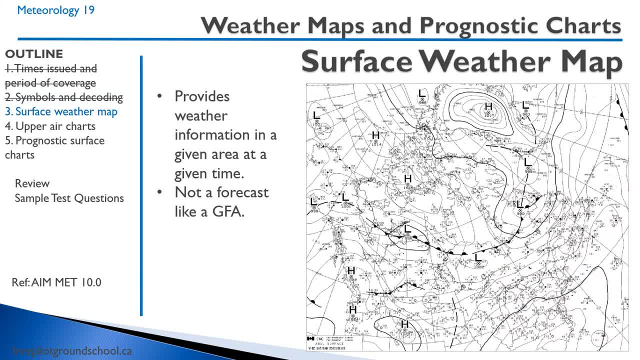 Here's an example of a surface weather map. It provides weather information at a given area at a given time. It's not a forecast like a GFA, It's just a weather map. It says: this is at this time, This is what was happening, So we can just look through here. We can see here: Here's a warm front going to a low. Here's the cold front. We have a high pressure region right here. 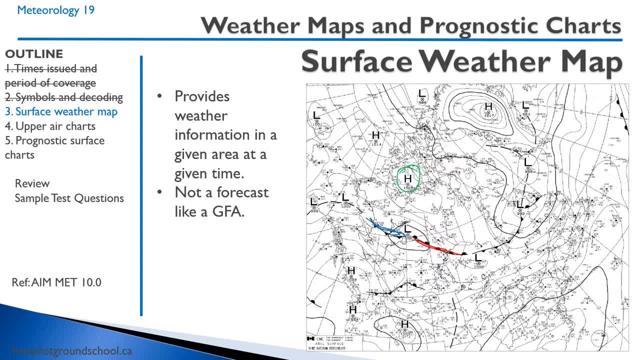 Here we have our isobars So we can look at it and we can roughly guess. this is kind of going to be what the weather is North America. if we're in Kansas, let's just say: or down here something. 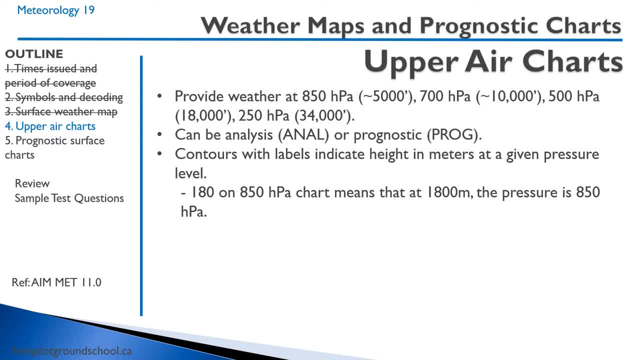 Upper air charts provide the weather at four different pressure levels. So this is kind of interesting. It's a bit different. So, remember, we normally have isobars and we say, okay, we're going to go to this. Okay, well, this is what the sea level pressure is at this location. What this does different is that it will say this is the pressure. The pressure is 850 hectopascals for this whole chart, But then it will give the altitude where it's 850 hectopascals or 700 or 500. Okay, so these go on pressure levels. These upper air charts can be analysis charts or prognostic. Prognostic is a forecast, Analysis is just the weather report. 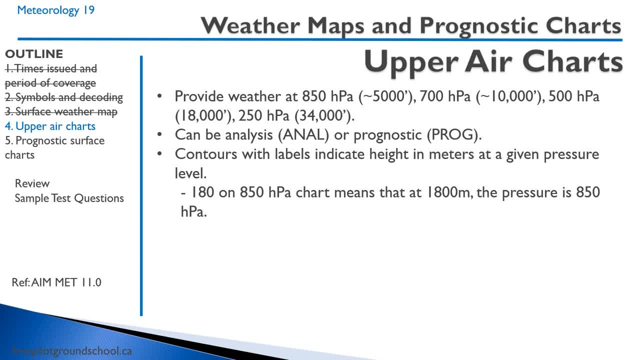 Outwears with labels indicate the height in meters at a given pressure level. So if we see 180 on the 850 hectopascals chart, that means that the height is 1800 meters where the pressure is 850 hectopascals. So kind of weird. I wouldn't put too much thought or effort into this, You just have to be aware of it. I have to teach it, But it's. it's pretty rare that you're actually going to look at this kind of chart. 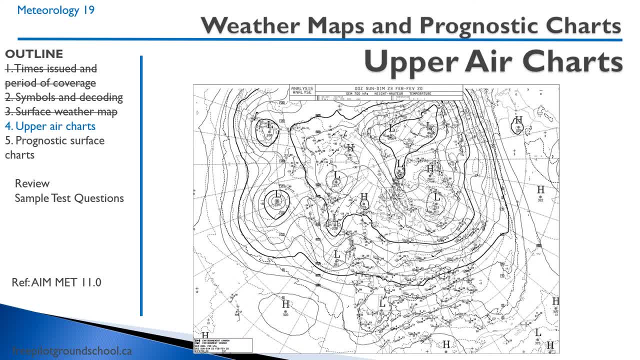 Okay. So here's an example. This is an analysis chart. So this is 700 hectopascals, So everything's going to be around 10,000 feet. That's what it kind of roughly works out to Okay. So here's a high. Okay, let's take a look: High 320.. So that means that this, the altitude, 3200 meters. At 3200 meters it's going to be 700 hectopascals. 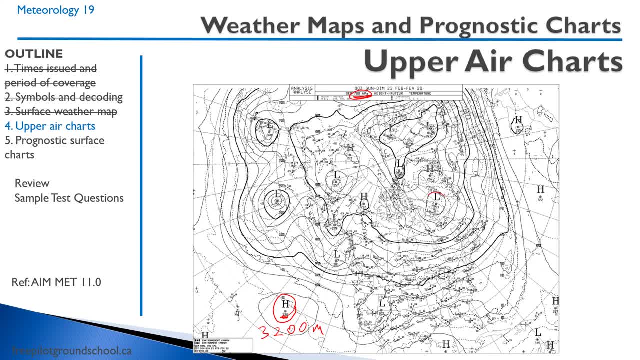 So let's look at another one Here: low 253.. Okay, So it's going to be 700 hectopascals at 2530 meters. So the lower, lower altitude, because it is because it's a low pressure region, So it's quite a bit different, but just be aware of it. 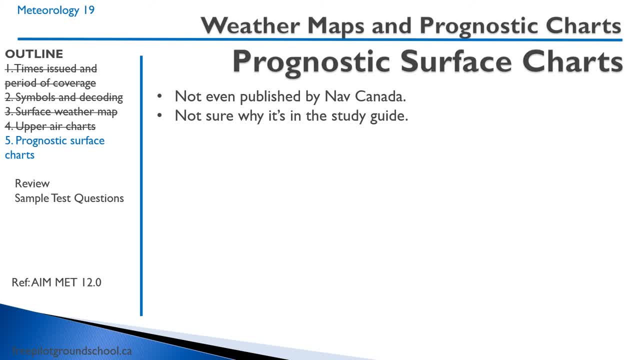 We have these prognostic surface charts and I have no idea what these are, what even these are. I couldn't find any information of these in any of my textbooks. They're not published by NAV Canada. I have no idea why it's in the study guide. 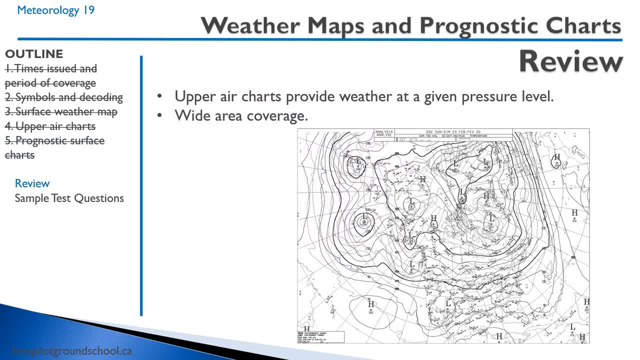 So this earns a useless step. Remember that upper air charts provide weather at a given pressure level. They are a wide area coverage Sample test question on the 700 hectopascal upper chart. So remember that's around 10,000 feet. What does 271 mean? So we see, right here, 271.. 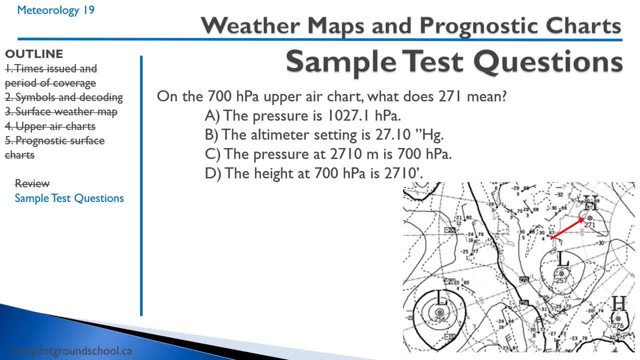 So remember, that's around 10,000 feet. What does 271 mean? So we see, right here, 271.. So we see, right here, 271.. So we see, right here, 271.. So remember, that's the altitude where the pressure is 700 hectopascals. 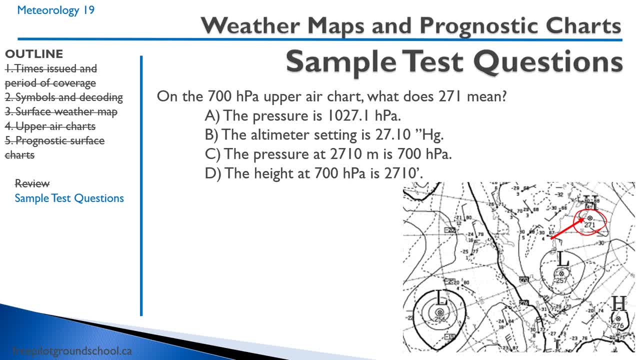 So that's 2710, because we had a zero on there. Correct answer C: the pressure at 2710 meters is 700 hector pascals. That concludes this lesson on weather maps and prognostic charts. Our next lesson is just going to be covering 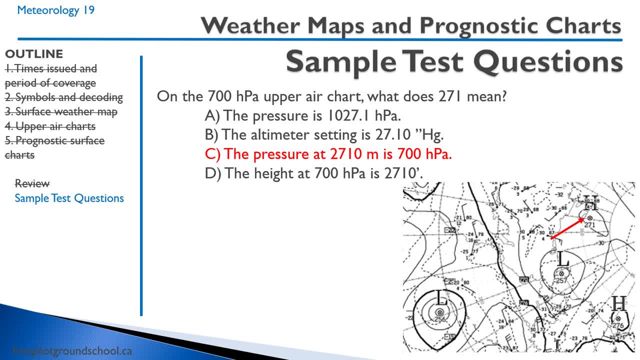 just working our way through some weather scenarios. Just working our way through some weather scenarios just for your practice, and we'll work on that next. Thanks for joining me and we'll see you at our next lesson.